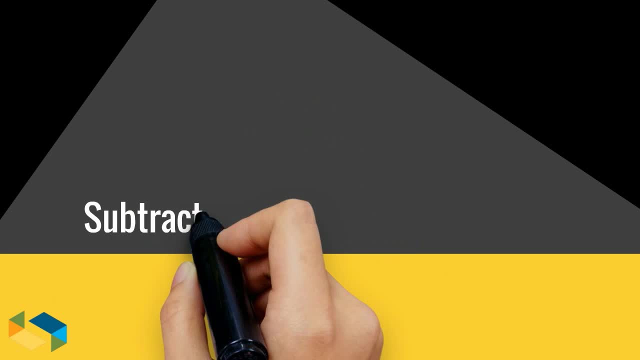 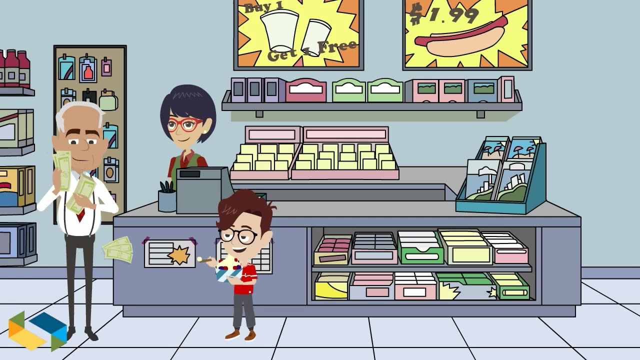 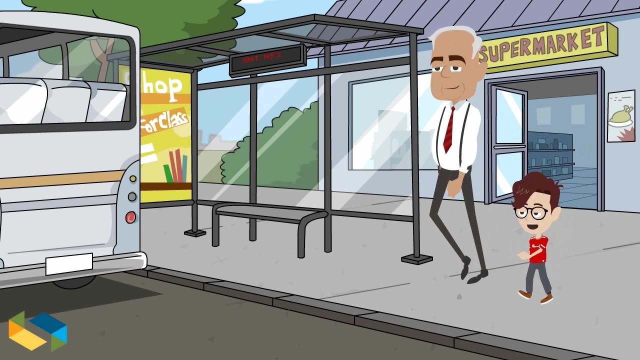 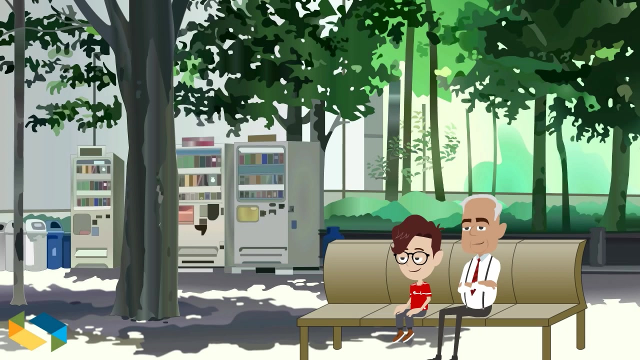 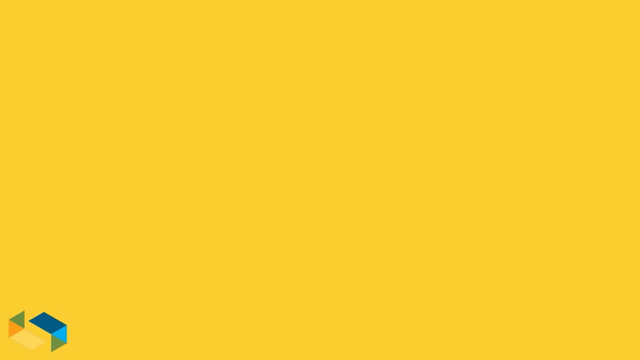 There is my change and we are done. Grandpa, can I ask you a question? Sure, son, How did you figure out how much change you get back after shopping? Oh, that's simple. We use subtraction. Can you explain what it means? Sure, Subtraction is the process of removing. 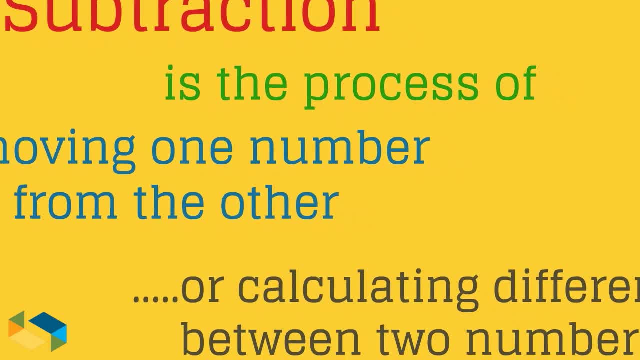 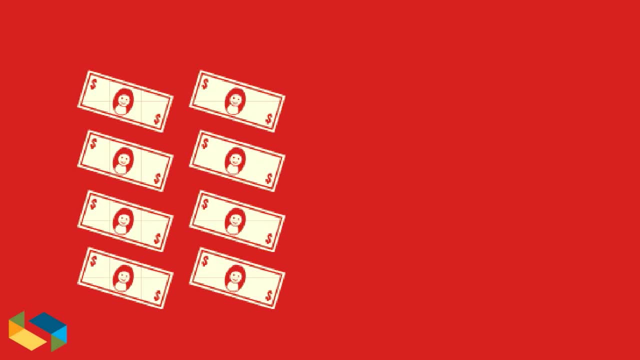 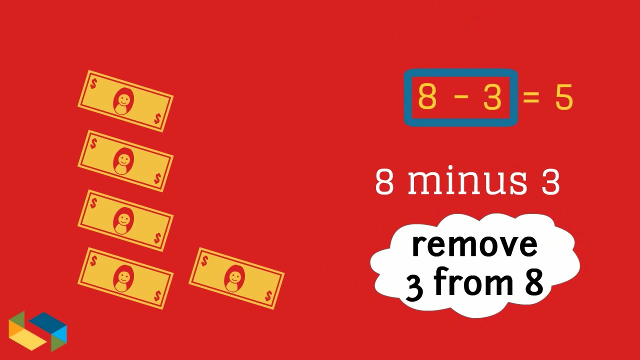 one number from another or calculating difference between two numbers. For example, let's say we have 8 currency bills and we spend 3. What we are left with are 5 currency bills. The subtraction expression is read as 8-3, which means to remove 3 from 8.. Here's how this. 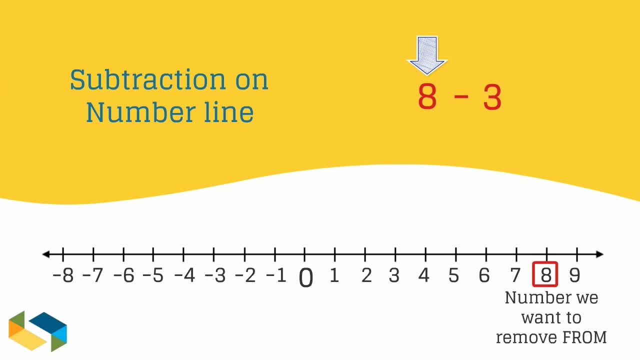 very problem is solved on a number line. We locate 8 on the line, the number we want to remove from. We move 3 spaces to the left as we are subtracting, Remember, in addition we move to the right, So subtraction is opposite of addition. Now we are at the number 5, which 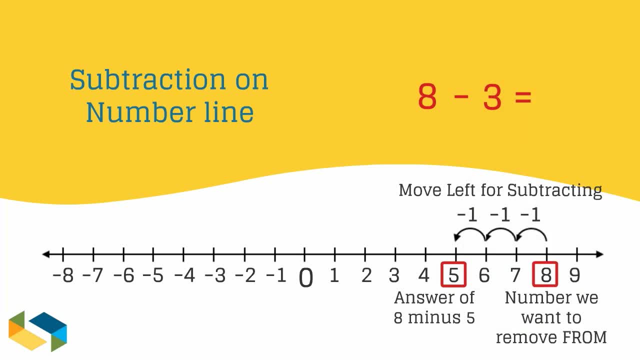 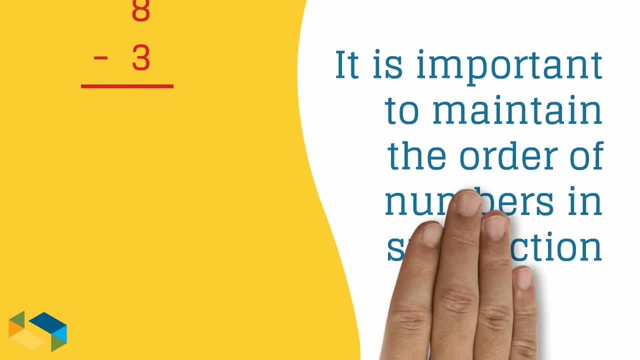 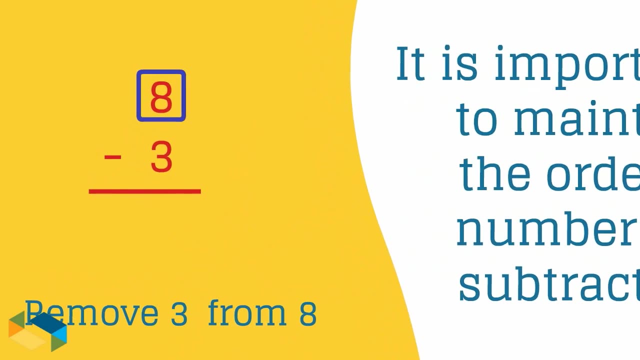 is the answer. So 8-3 is 5.. You have to remember that in subtraction the order of numbers is very important. Taking the same example, there is a certain way 8-3 is to be written. You place the bigger. 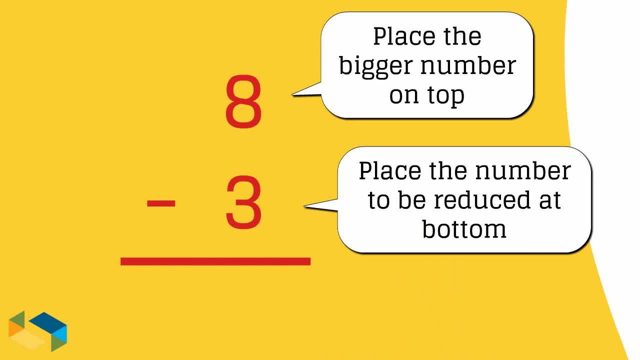 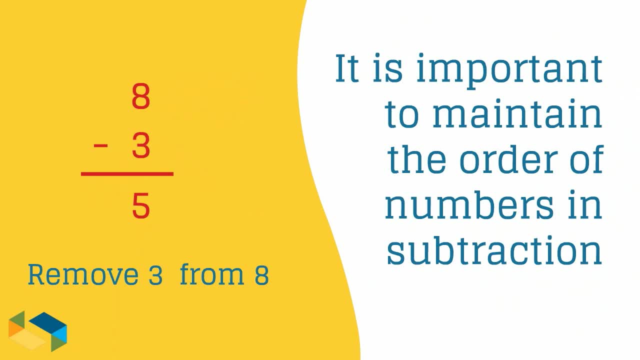 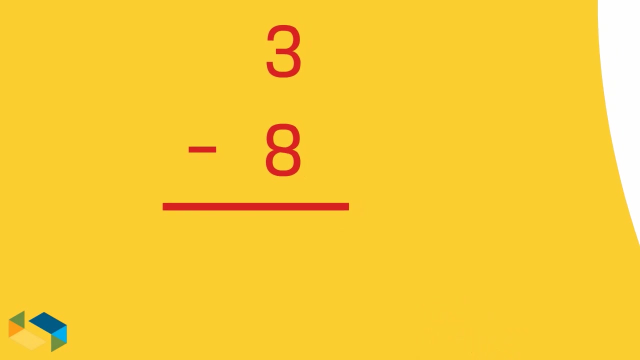 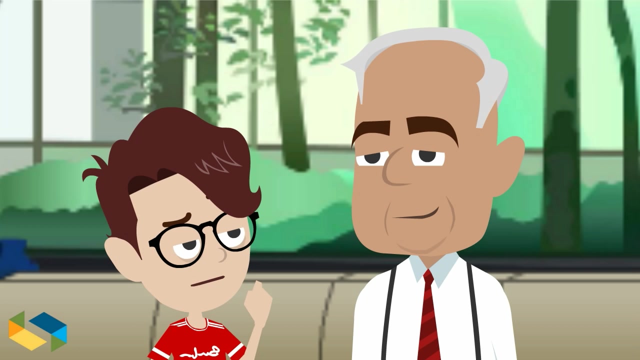 number at the top and the number to be reduced at the bottom. The answer, of course, is 5, as we saw earlier. However, if we interchange the order of writing these numbers, the answer doesn't hold true. The answer for 3-8 is 5, for the matter of fact. 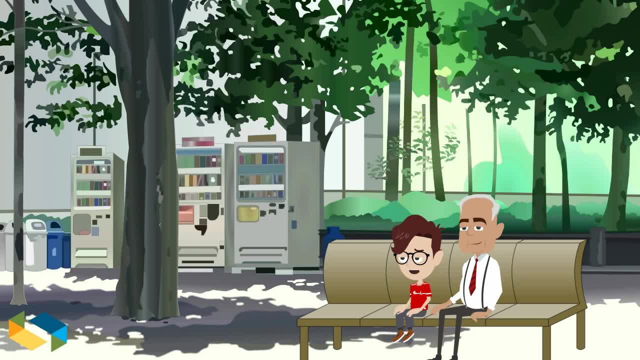 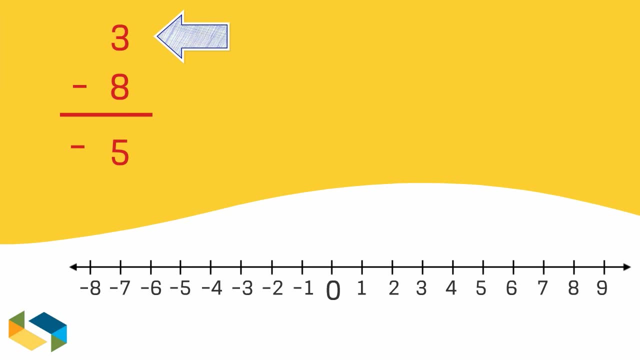 But, grandpa, How can we remove 8 from 3?? Isn't it impossible? Good question, Let's check this out. on number line, We locate 3. number we need to remove from. We go 8 spaces to the left and we get the answer as minus. 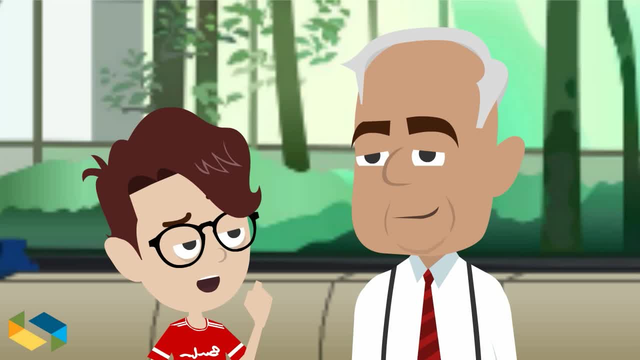 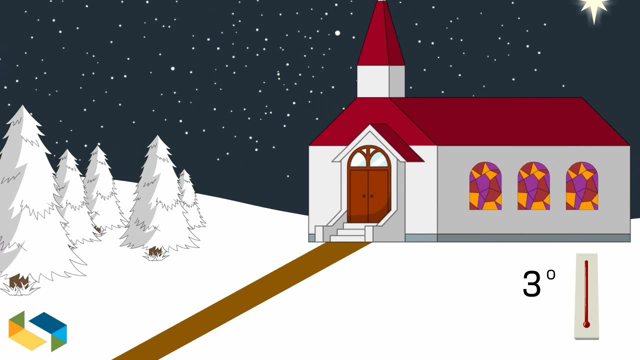 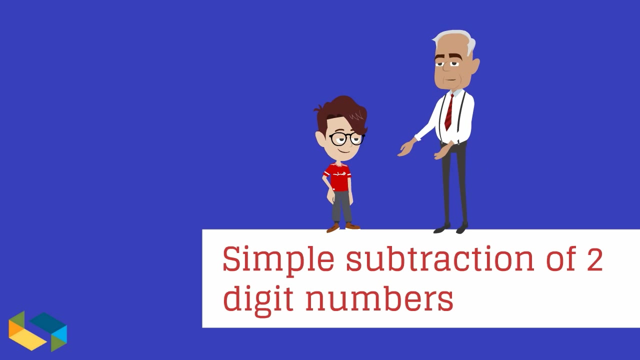 5.. But is there a real world situation to describe this? Suppose there are very chilly conditions and the temperature is at 3 degrees. With a snowstorm coming, the temperature drops by 8 degrees to minus 5.. Now, son, let's look at another simple example of subtraction. 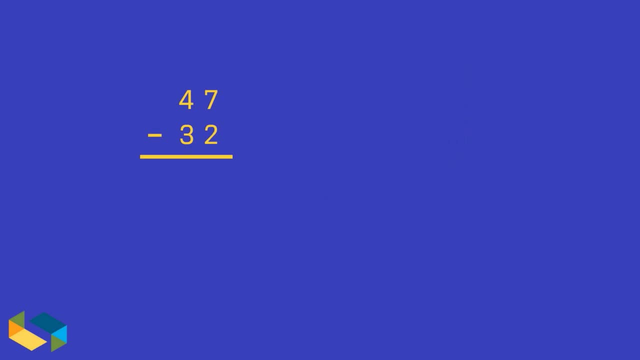 this time with 2 digit numbers, say 47 minus 32,, which is to check what remains after we remove 32 from the number 47. We start at the 1 space. Here we have 7 minus 2, which means to remove 2 from 7.. 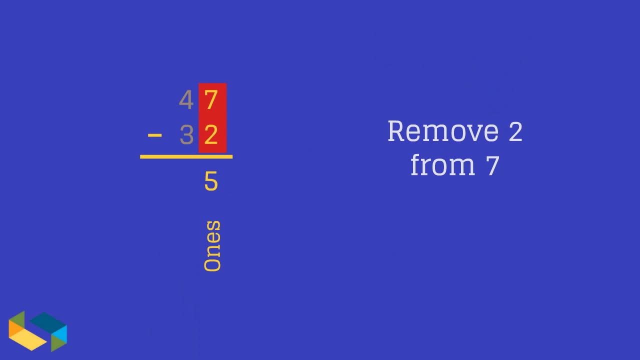 Subtraction, Subtraction, Subtraction. The answer for the 1 space is 5.. Now we move to the 10th place, where we have to remove 3 from 4.. The answer, of course, is 1.. So the answer of 47 minus 32 is 15.. 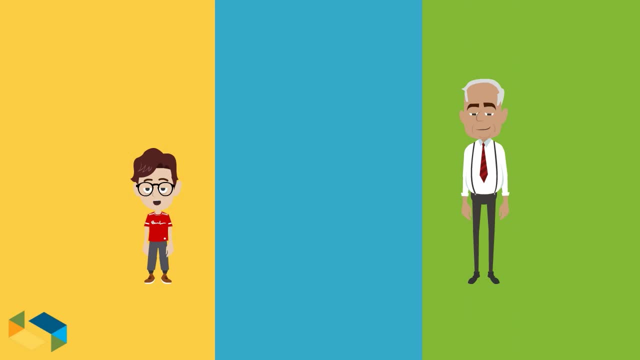 Grandpa, can you describe where in our day to day life is subtraction used? Sure, son, Basically, there are 3 different types of situations in real life where we frequently use subtraction. Let's look at them. Firstly, subtraction is used when we 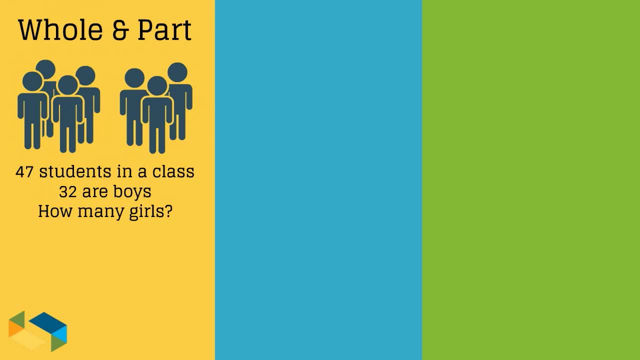 have to identify a part from a whole. Say 47 students in a class, 32 of them are boys. How many are girls? As we calculated before, the answer is 15 girls. Another example is subtraction, Subtraction, Subtraction. 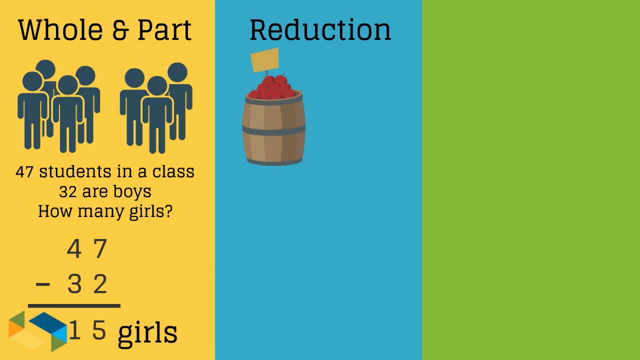 Subtraction, Subtraction. Another situation where subtraction is used is when we have to reduce or decrease something. For example, we give away 32 apples from 47 apples. What remains with us? We use subtraction to find out the answer, which is 15 apples.